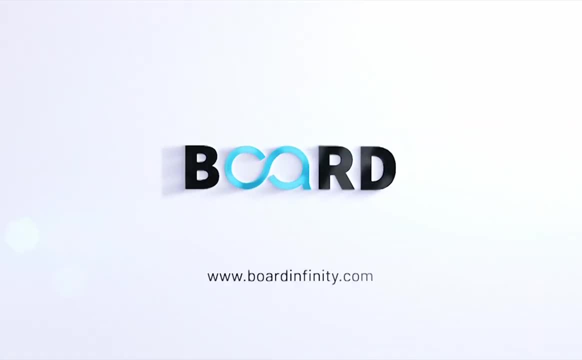 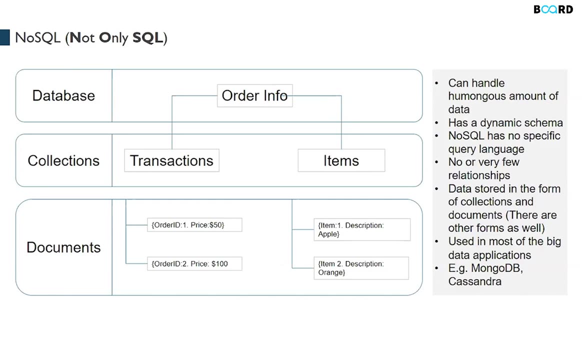 What is NoSQL? NoSQL generally stands for not only SQL, which means anything you know, not in a tabular structure is the database name is given as not only SQL. right, okay, because as and when the data became more complex, so just imagine, every day the digital landscape is changing so much that 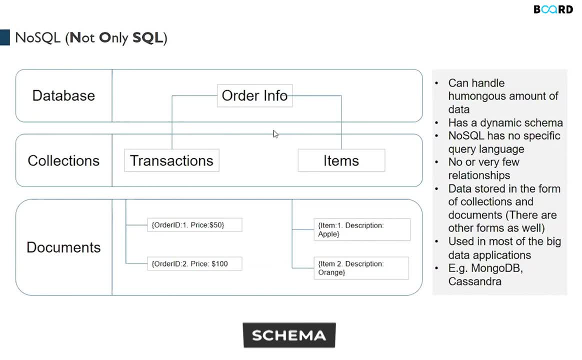 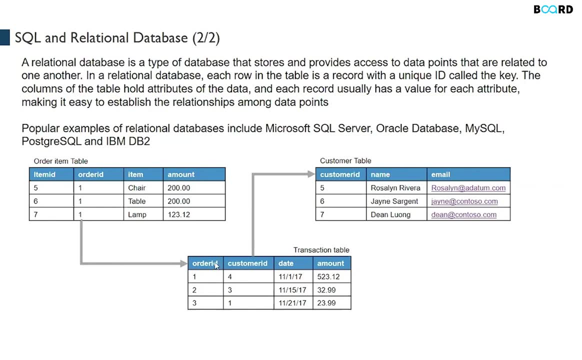 you cannot have a fixed schema. so what I? what do I mean by schema? schema means this: right, I've defined that order item will always have four columns, customer will always have three columns, transaction will always have four columns. that's a schema that I've defined. but you can't expect 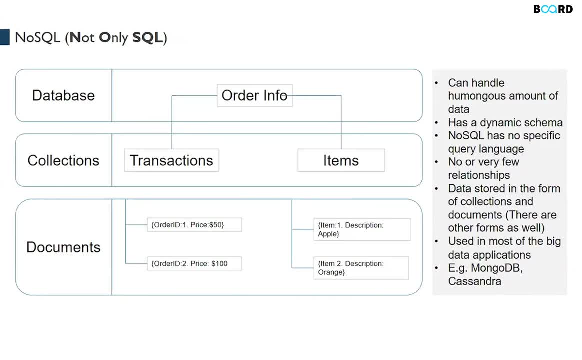 it in today's world. today it will be something, tomorrow it will be changed to something right. so these- not only SQL databases- have a dynamic schema. that means you can keep changing your schema. importantly, NoSQL has no specific query language. like SQL, there are different languages for different kinds of NoSQL database. this is just one form of storage of data. this is 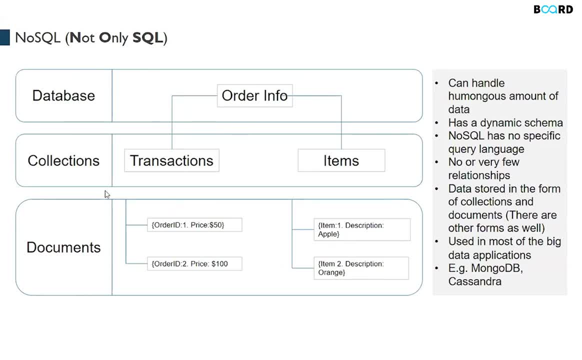 called the collection and documentation form, but there are other forms as well. in NoSQL there is a graph database, there's a key value column pair, a lot of things right now. this is very, very new in the industry, not only SQL. very new means means relatively new. okay, NoSQL and SQL supports. 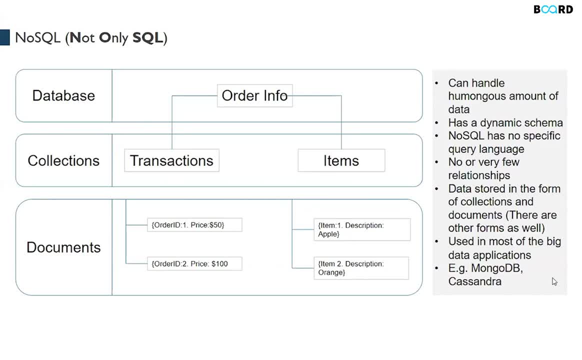 everything. SQL also supports audio and video storage. so NoSQL also supports audio and video storage. so NoSQL also supports audio and video storage. so NoSQL also supports audio and video storage. but the main difference is SQL databases store relationships in the form of tables- NoSQL. 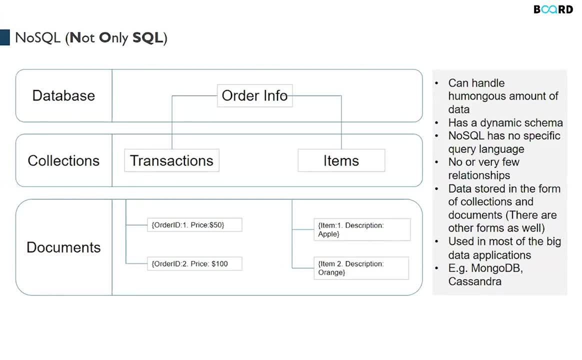 does not solve. store it in the form of tables it. it stores it in the form of key value pairs. it stores it in the form of a graph database. so what I would advise you to do is I will share this material with you now. any company- right you can see, Amazon, or Facebook or Microsoft- has both, because 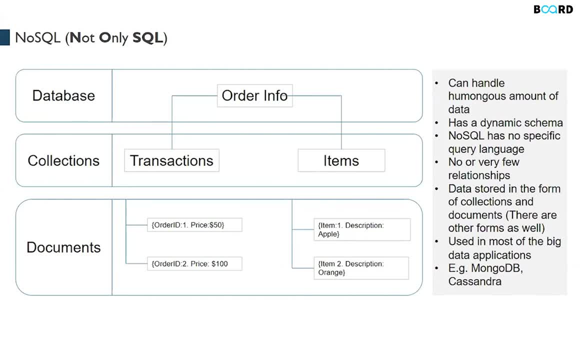 relational database has its own advantage. non-relational database also has its own advantage. so usually what you can do is you can create a database and then you can create a database. so usually what you can do is you can create a database and then you can create a database. 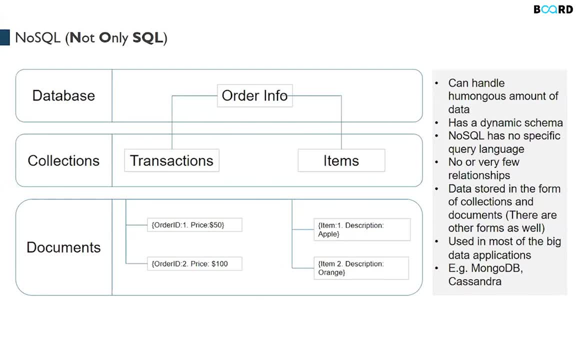 you see is it's a mixture of both databases, the company will have. what I you see is it's a mixture of both databases, the company will have. what I you see is it's a mixture of both databases, the company will have. what I want you to do is go back. 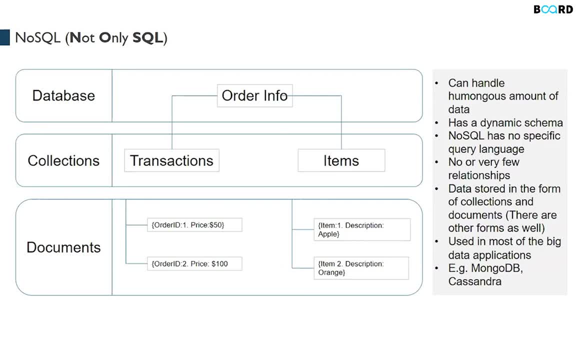 want you to do is go back. want you to do is go back research as much as you can about you know research as much as you can about you know research as much as you can about you know NoSQL database and have a good at least NoSQL database and have a good at least. 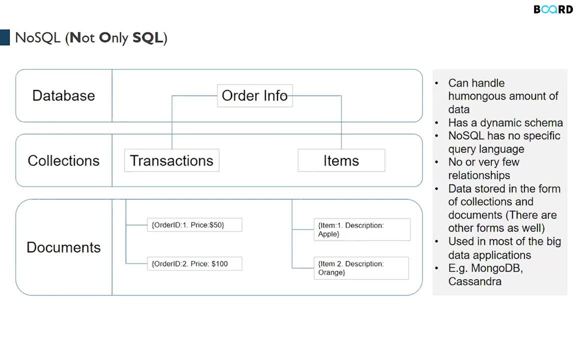 NoSQL database and have a good, at least knowledge of having, like you know, a knowledge of having, like you know, a knowledge of having, like you know, a discussion. if someone asks, hey, do you know discussion? if someone asks, hey, do you know discussion? if someone asks, hey, do you know NoSQL, you can say, yes, I know what. 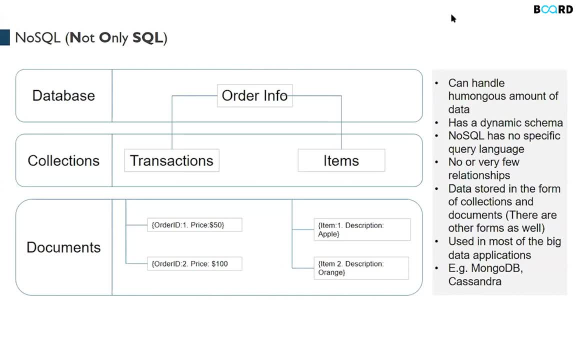 NoSQL. you can say: yes, I know what NoSQL. you can say, yes, I know what NoSQL is and you can have the discussion. NoSQL is and you can have the discussion. NoSQL is and you can have the discussion. right, I have listed down some differences. 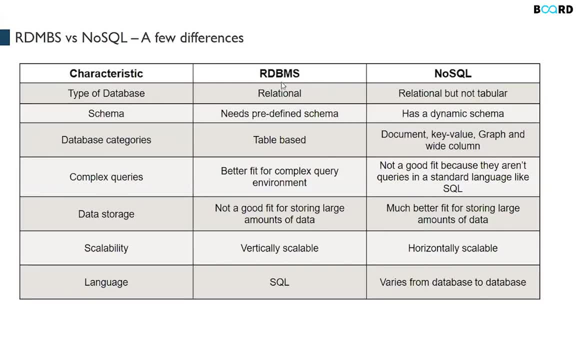 right, I have listed down some differences. right, I have listed down some differences which can be useful for you. type of which can be useful for you. type of which can be useful for you. type of database: our DBMS is relational NoSQL database. our DBMS is relational NoSQL. 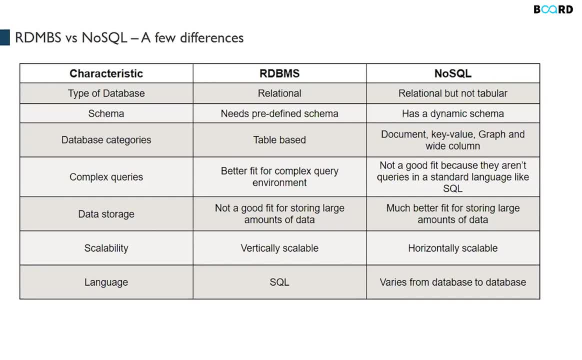 database, our DBMS, is relational NoSQL. now, if you look at the internet and most now if you look at the internet and most now if you look at the internet and most of the blocks or whatever information of the blocks or whatever information of the blocks or whatever information they, they say that NoSQL is not. 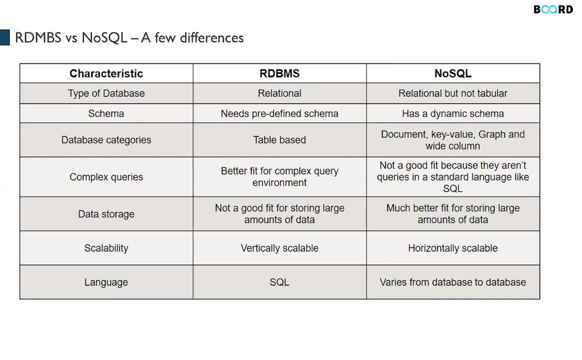 they say that NoSQL is not. they say that NoSQL is not relational, which is actually not true. okay, relational, which is actually not true. okay, relational, which is actually not true. okay, NoSQL also has relationship between NoSQL, also has relationship between NoSQL. also has relationship between different pieces of information. so what I 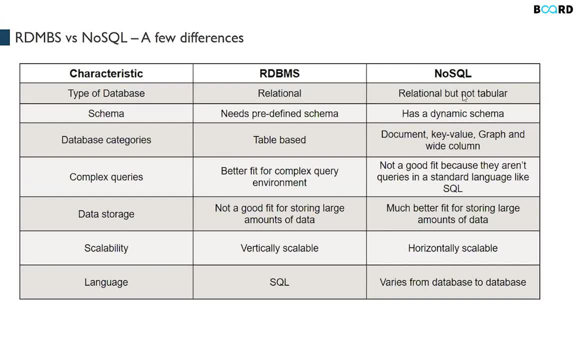 different pieces of information, so what I different pieces of information, so what I would call it is. it is relational, but would call it is. it is relational but would call it is. it is relational but it is not tabular. okay, because I've seen it is not tabular. okay, because I've seen. 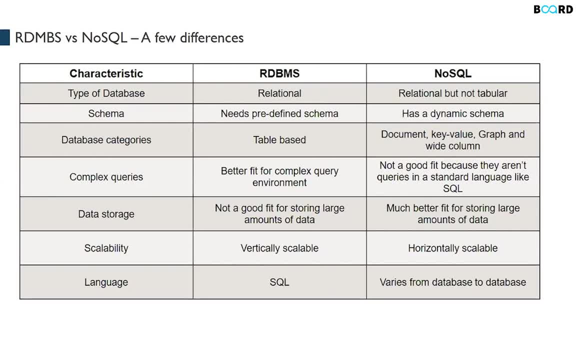 it is not tabular, okay, because I've seen this common misconception among this common misconception, among this common misconception among different people saying that a most different people saying that a most different people saying that a most equal means no relation, which is wrong. equal means no relation, which is wrong. 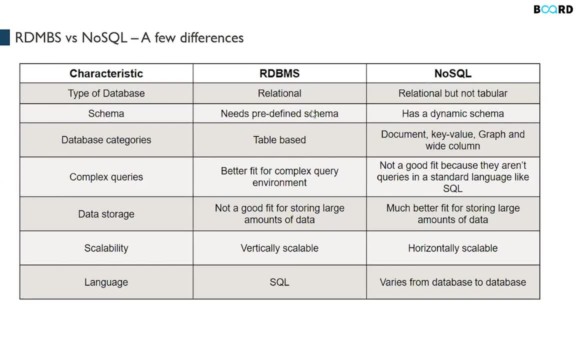 equal means no relation, which is wrong. okay, schema: it needs a predefined schema. okay, schema, it needs a predefined schema. okay, schema, it needs a predefined schema. like I said, NoSQL does not need a. like I said, NoSQL does not need a. like I said, NoSQL does not need a predefined schema. these are the database. 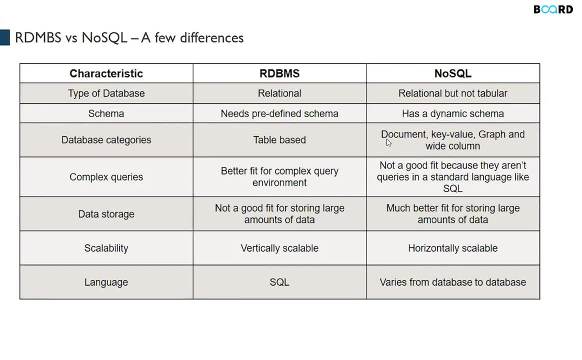 predefined schema. these are the database predefined schema. these are the database categories are talking about right. this categories are talking about right. this categories are talking about right. this is table based. this is document. it can is table based. this is document. it can is table based. this is document. it can be document based, like we saw here, right. 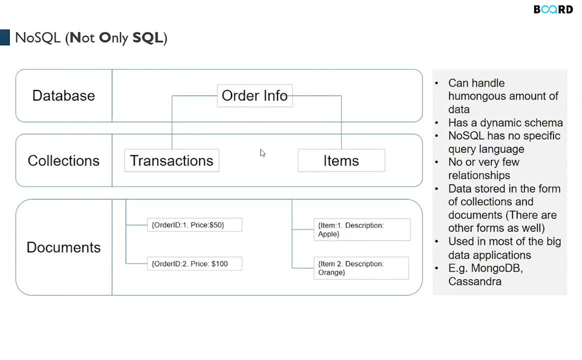 be document based, like we saw here right. be document based like we saw here right. let's say there are two. there is an. let's say there are two, there is an. let's say there are two. there is an order info. there is transaction and item order info. there is transaction and item. 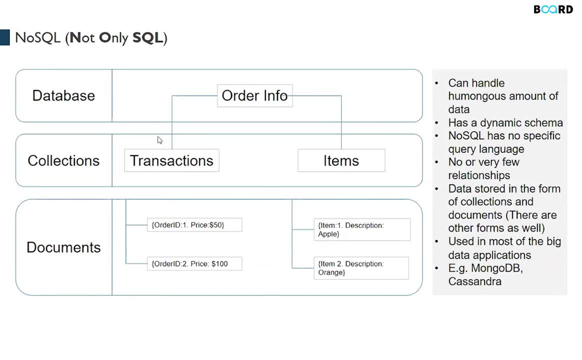 order info. there is transaction and item order in first transaction item. so order in first transaction item. so order in first transaction item. so this these fields instead of tables. it will this these fields instead of tables. it will this these fields instead of tables. it will go to something called as connection. 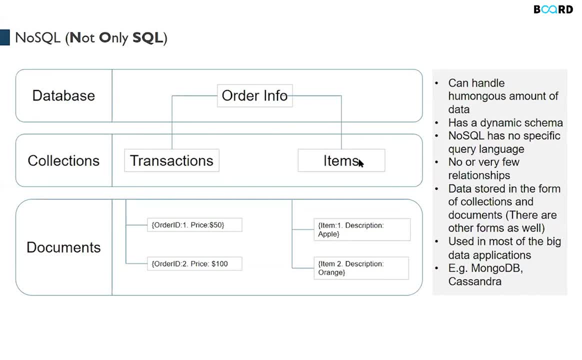 go to something called as connection. go to something called as connection in our relational database. this would be in our relational database. this would be in our relational database. this would be one table. this would be another table. one table. this would be another table. one table. this would be another table. after collection. it will go to the 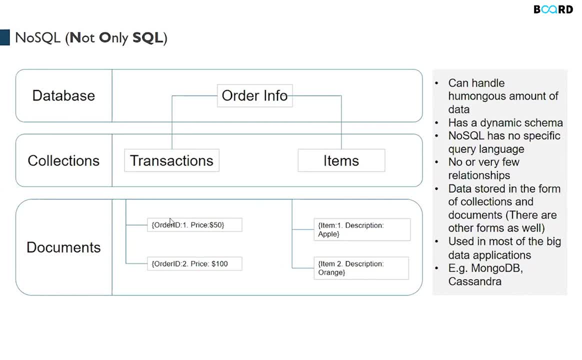 after collection. it will go to the after collection. it will go to the information that is stored, will go to information that is stored, will go to information that is stored, will go to something called document. okay, that's something called document. okay, that's something called document. okay, that's how. if let's say, you know, if you talk, 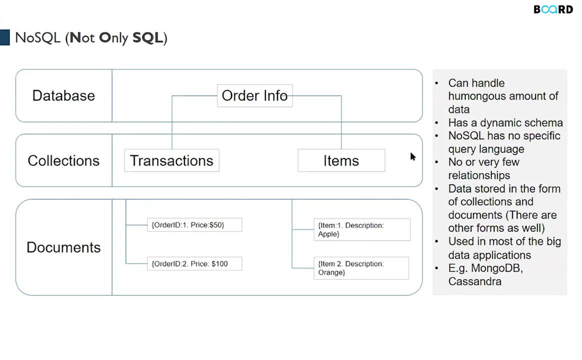 how. if let's say: you know if you talk how. if let's say you know if you talk about no sequel, that's how it will be about no sequel, that's how it will be about no sequel. that's how it will be stored. now, if there is a new, new piece. 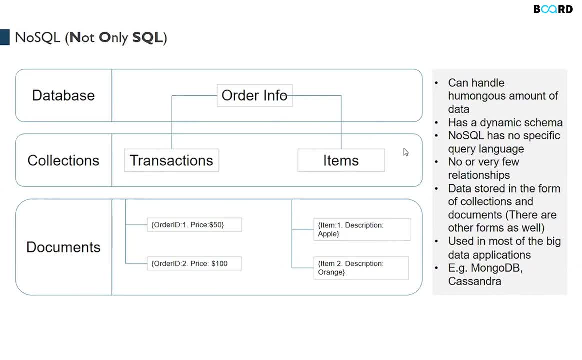 stored now if there is a new new piece stored now. if there is a new new piece of information, there will be a new of information. there will be a new of information. there will be a new collection in this order. info without collection in this order. info without: 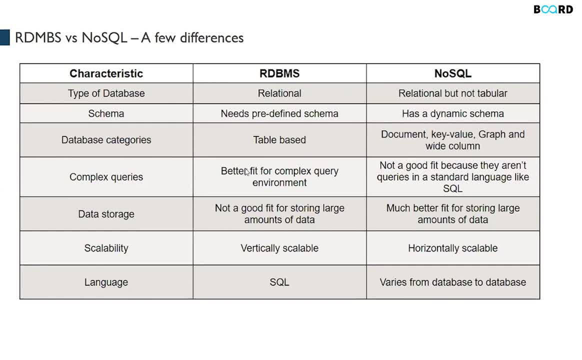 collection, in this order: info without much change in the schema: complex, much change in the schema. complex, much change in the schema. complex. queries now relational database is a queries now relational database is a queries. now relational database is a better fit for complex query. okay, like i. better fit for complex query. okay, like i. 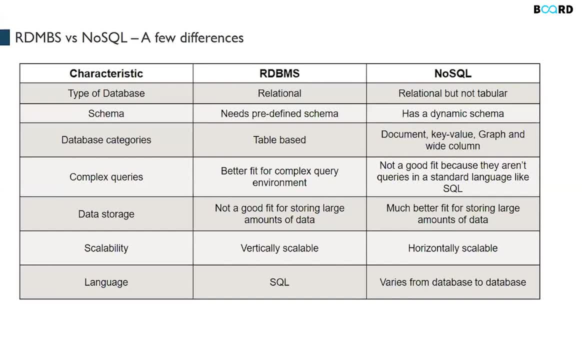 better fit for complex query. okay, like i said, both relational database and no said. both relational database and no said. both relational database and no sql database have their own advantage and sql database have their own advantage and sql database have their own advantage and disadvantage. one of the main advantage: 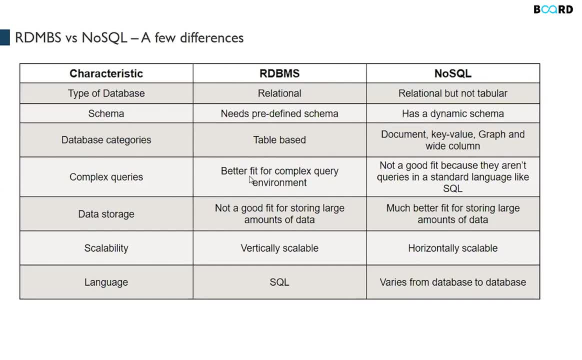 disadvantage one of the main advantage, disadvantage one of the main advantage of relational databases. it is very easy of relational databases. it is very easy of relational databases. it is very easy to write a piece of code on relational. to write a piece of code on relational. to write a piece of code on relational database- no sql, it is a little bit. 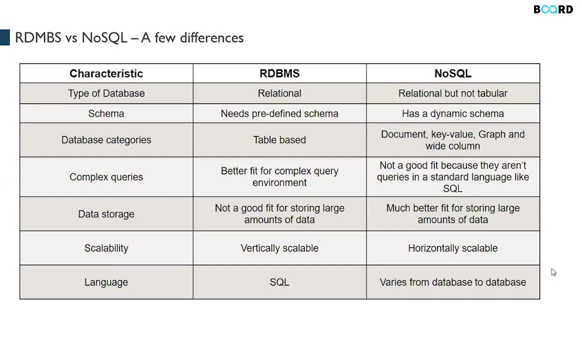 database- no sql. it is a little bit. database- no sql. it is a little bit difficult because there are different. difficult because there are different. difficult because there are different languages for different. uh, you know no languages for different. uh, you know no languages for different. uh, you know no sql. data storage- again, it is not a good. 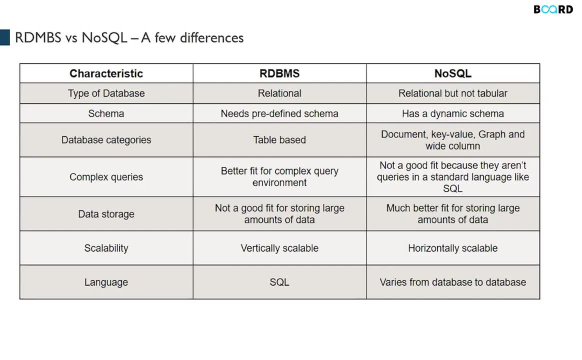 sql data storage. again. it is not a good sql data storage. again, it is not a good fit for storing large amounts of data. fit for storing large amounts of data. fit for storing large amounts of data because it tends to get little heavy. and because it tends to get little heavy and. 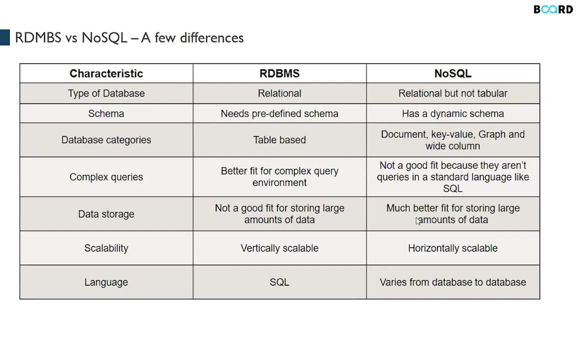 because it tends to get little heavy and slow. uh, since it is rigid, no sql is it's slow. uh, since it is rigid, no sql is it's slow. uh, since it is rigid, no sql is. it's a much better fit for storing large. a much better fit for storing large. 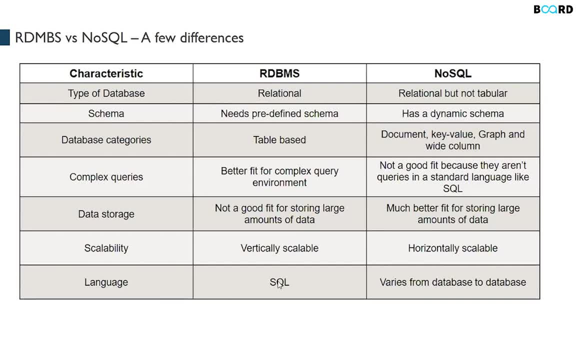 a much better fit for storing large amount. scalability: vertically scalable amount scalability: vertically scalable amount. scalability: vertically scalable horizontally. language: here sql is used horizontally. language here sql is used horizontally. language: here sql is used. no sql. it just varies from database to no sql. it just varies from database to. 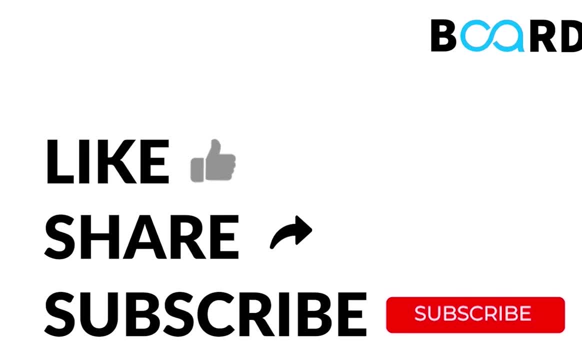 no sql, it just varies from database to database, database database. there is no fixed language. 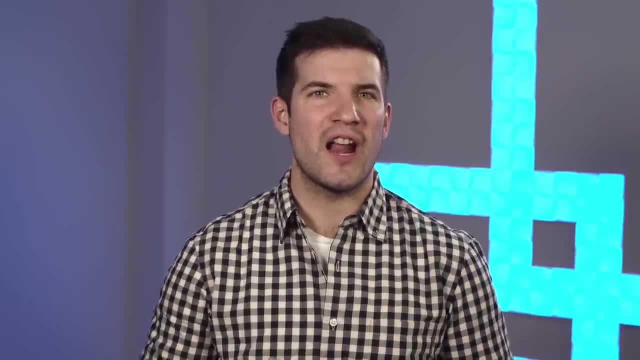 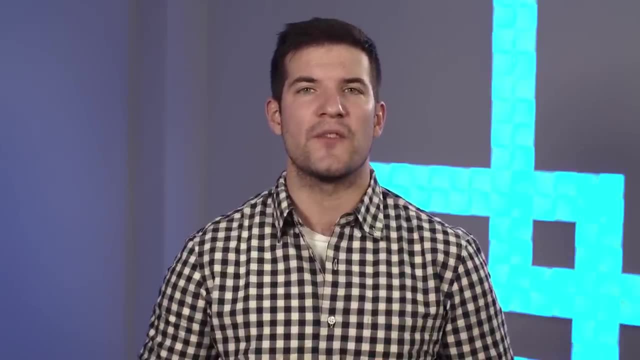 Welcome to our data analysis with Python tutorial. My name is Santiago and I will be your instructor. This is a joint initiative between FreeCodeCamp and Remoter. In this tutorial, we'll explore the capabilities of Python and the entire PyData stack to perform data analysis. We'll learn how to read. 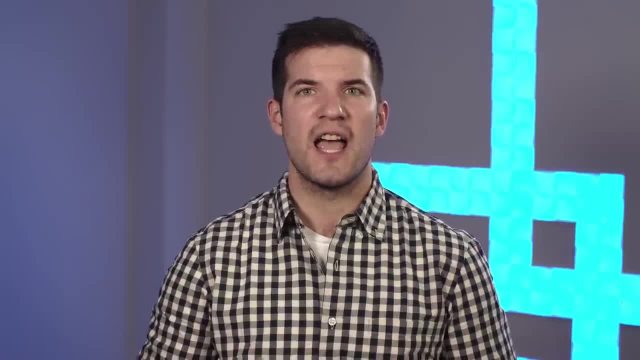 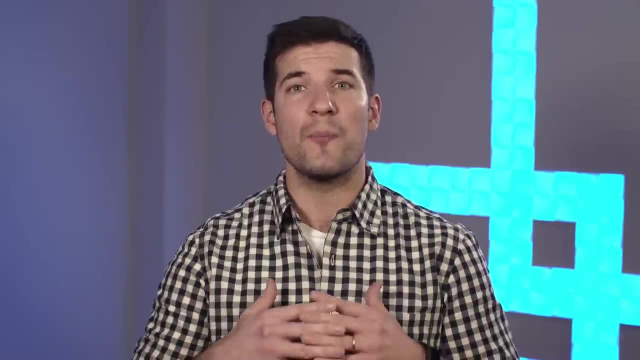 data from multiple sources, such as databases, CSV and Excel files, how to clean and transform it by applying statistical functions and how to create beautiful visualizations. We'll show you all the important tools of the PyData stack: Pandas, Matplotlib, Seaborn and many others. This 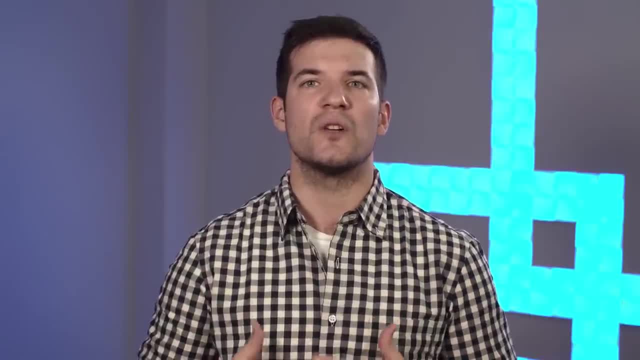 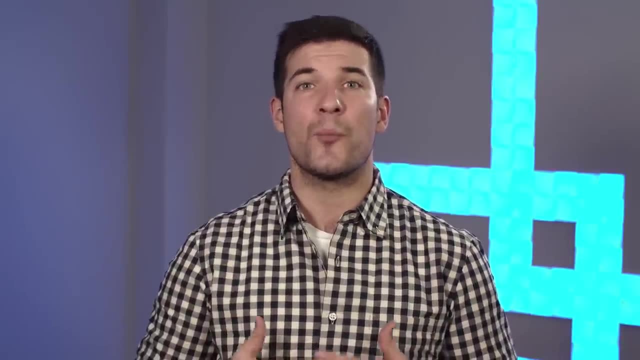 tutorial is going to be useful both for Python beginners that want to learn how to manage data with Python and also traditional data analysts coming from Excel Tableau, etc. You'll learn how programming can power up your day to day analysis. So let's get started.